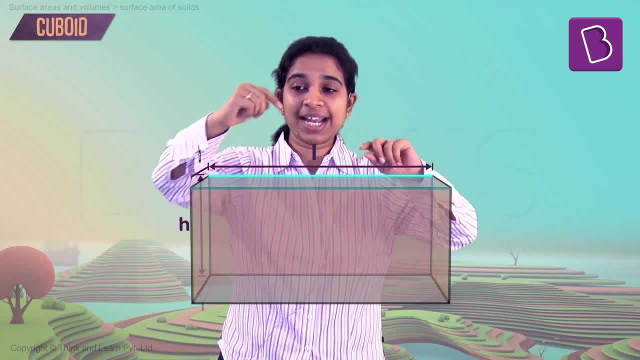 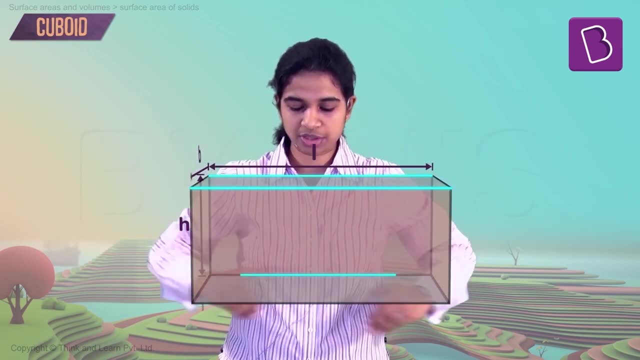 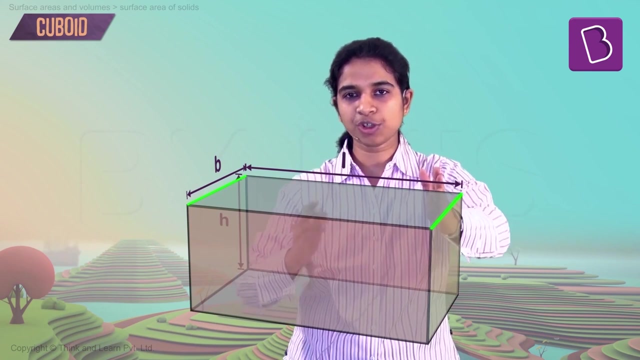 Now, if this length is L, you will notice that these 3 other edges also have length L, So these 4 edges will be L: 1, 2, 3 and 4.. All 4 will be L. Similarly, if this edge is B, you will have this also B, this also B and this also B. So you have 4 Bs. we have 4 Ls, 4 Bs. 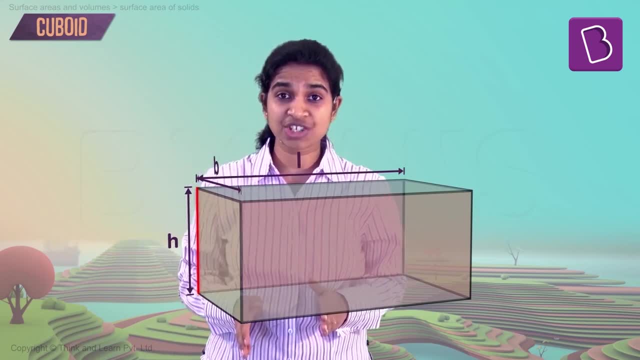 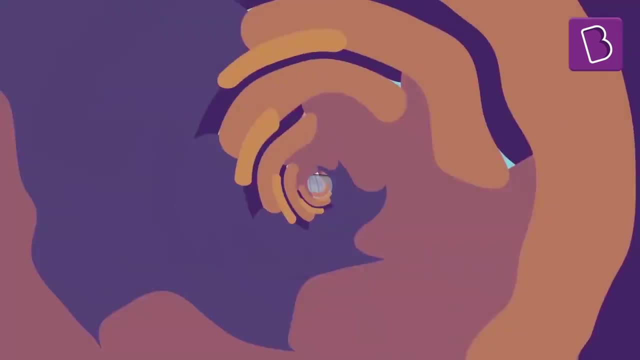 Similarly, if this edge is H, this will be H, this will be H. So we have 4 Ls, 4 Bs and 4 Hs. If we now open the cuboid up, this is what we will have. 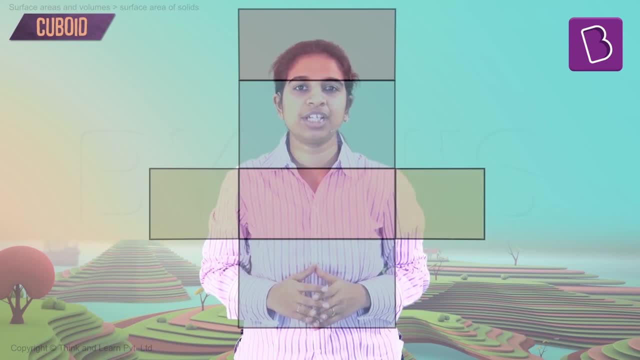 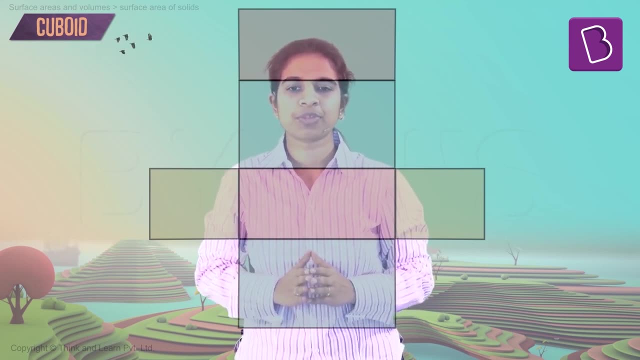 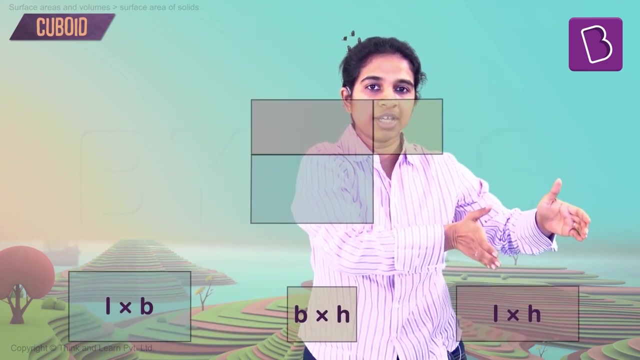 What you see here is 6 rectangles. We can now, using these 6 rectangles, very easily determine what the area of the cuboid is going to be. This is L x B. this is B x H. this is L x H. Now, similarly, you see there is one more of each of these types. 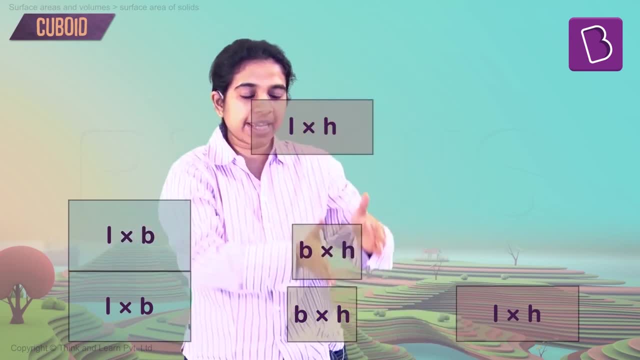 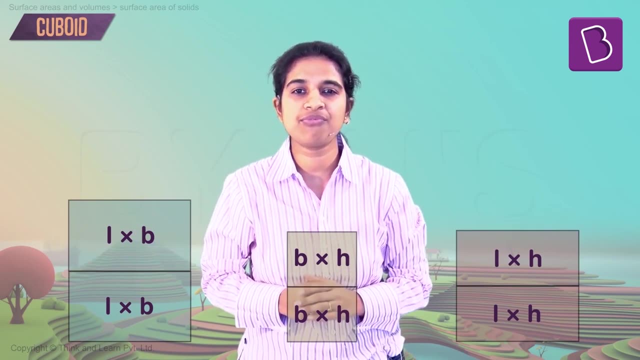 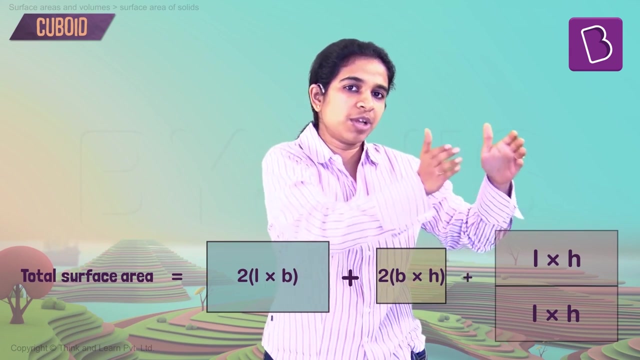 So this is the second L x B, this is again B x H and this is again L x H. We have all of the 6 rectangles here Now. if we add everything up, the area we will get is 2 x L x B plus 2 x B x H plus 2 x L x H. 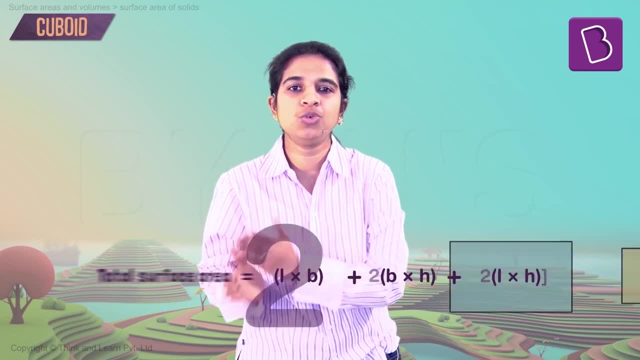 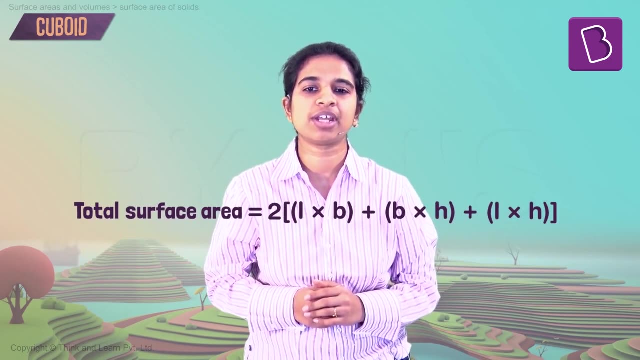 That's the total surface area of a cuboid: 2 x L x B plus B x H plus L x H. That's all You now know, the formula for total surface area of a cuboid. If you were now instead asked the lateral surface area, 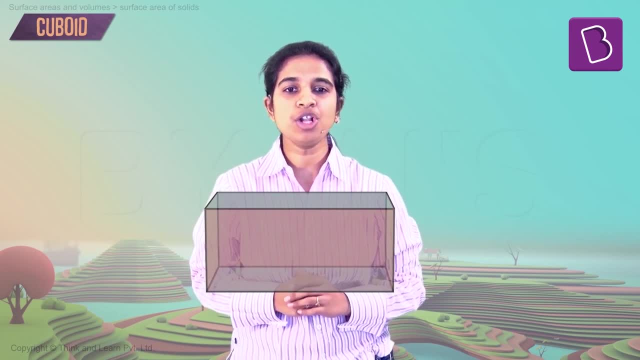 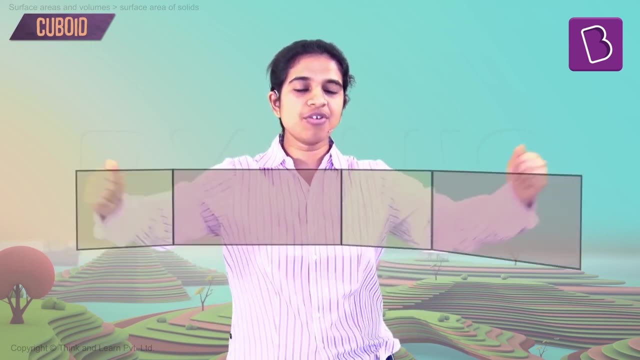 The same cuboid. you were asked the lateral surface area. All you need to do is remove the top and the bottom surface, Because lateral surface area is area of the sides. Now, if you open this up, we are left with only 4 rectangles. 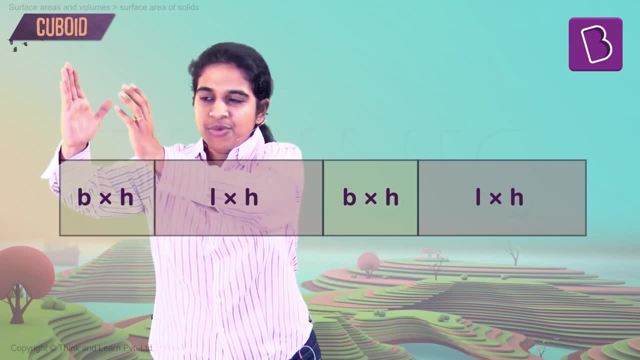 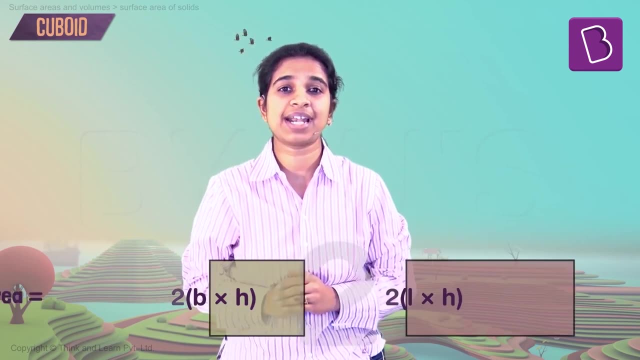 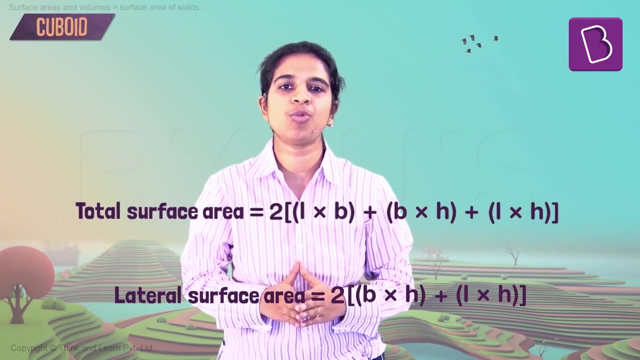 The 2 L x B rectangles are missing. So now we have B x H 2 of these and L x H 2 of these. That is the lateral surface area. 2 x B x H plus L x H. Those are the 2 areas of a cuboid.